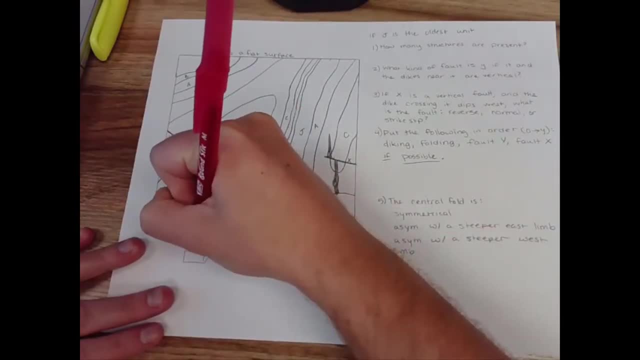 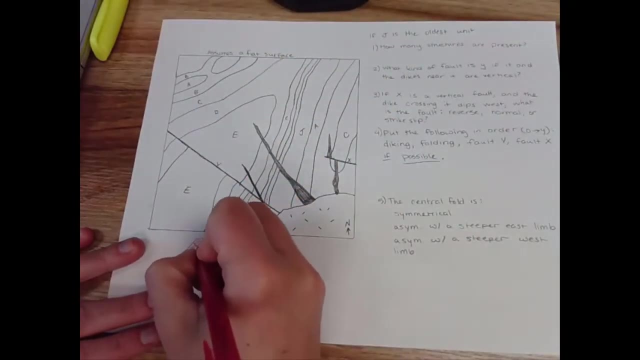 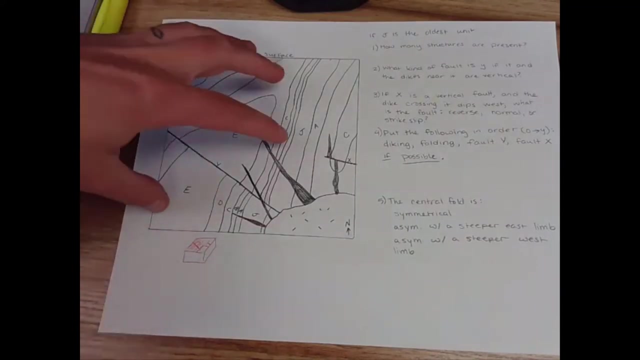 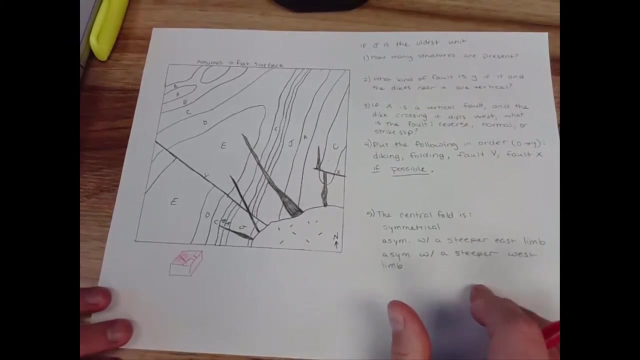 that in the surface you've got kind of this, this type of situation, so that's kind of what your surface looks like, but it's totally flat, okay. so this is just on here, but then we're going to answer a series of questions about this. so the 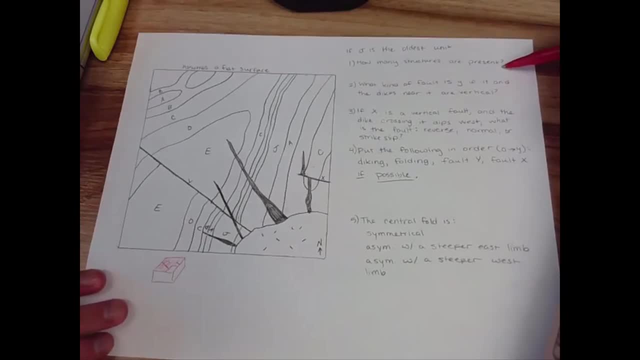 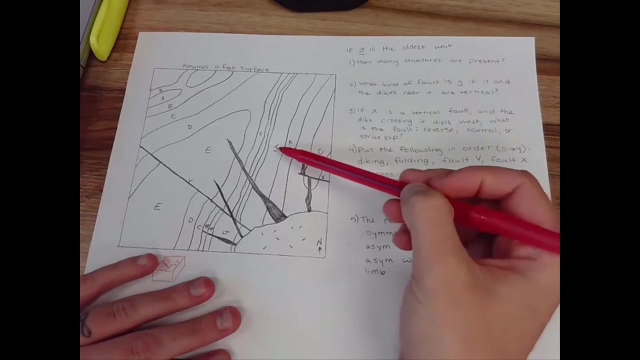 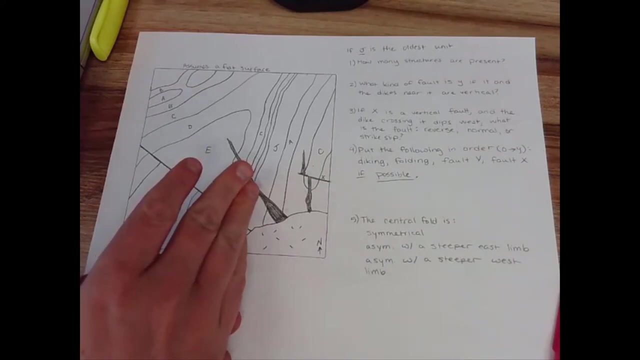 first question is how many structures are present, and we're going to also identify what they are. so we know that J is the oldest unit, so let's go find J. here's J, and if J is the oldest unit, then let's see we've got a than a blank. 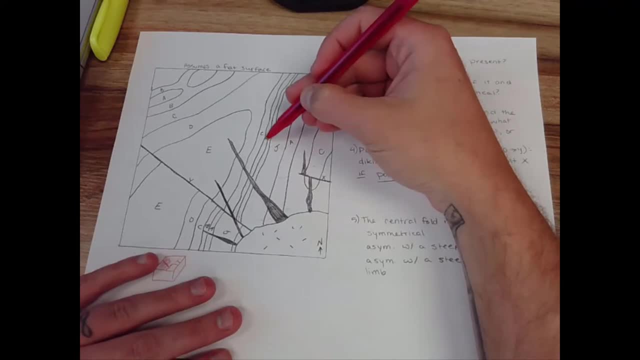 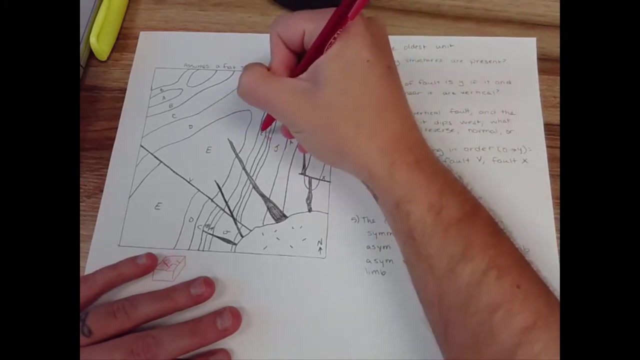 then C. then on this side we've got blank, blank C, so I'm gonna go ahead and start filling in units that aren't labeled. if this is a and there's two blanks in a, C, then this is ABC, this is J, a, B, C, this must be D, then you have E and we go back. 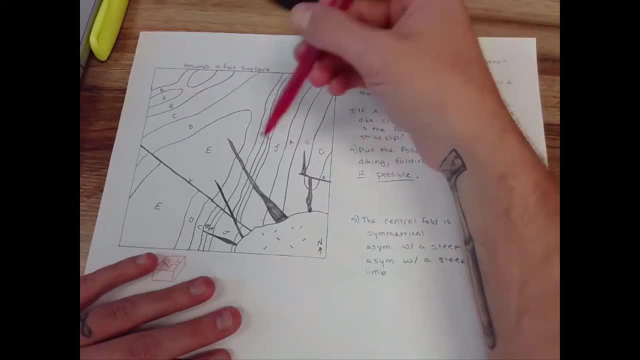 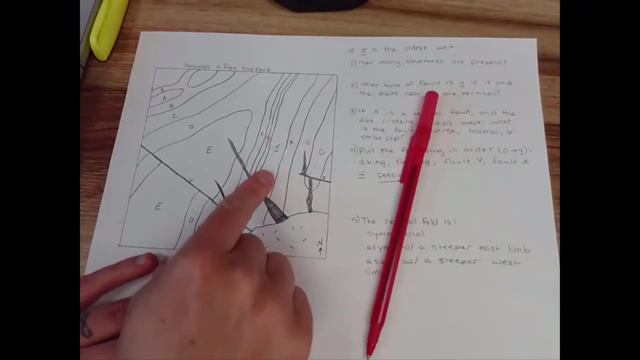 toward a, but we don't hit J again, okay. so let's think about what structures we have here if J is really old, but it's only exposed at this point and you've got a on this side, and on this side of it a has to be above J. so I'm just gonna 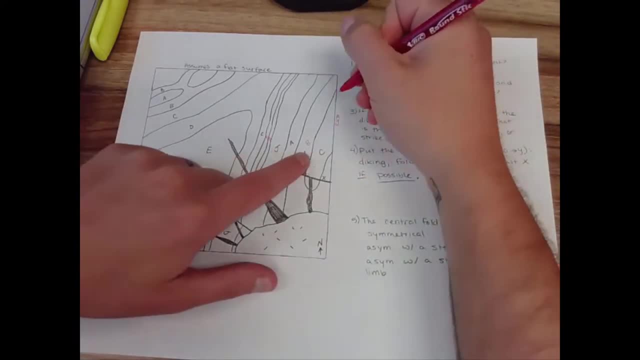 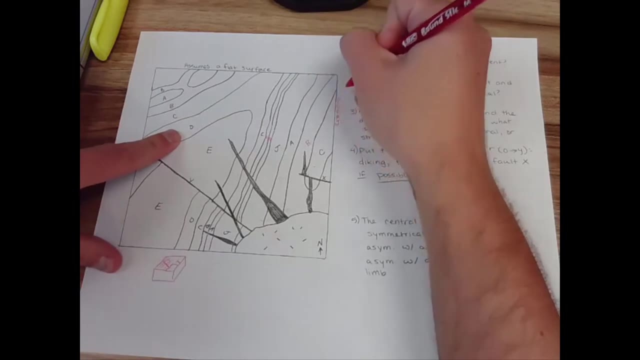 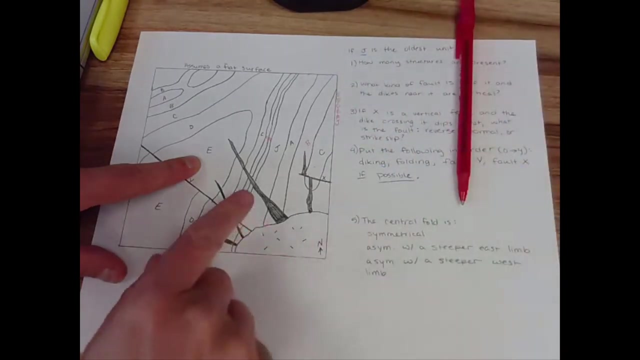 write out a little stratigraphy for myself: a, then B, then C, then over here, D e. ok, so I've got J, a, B, C, D, e, where e is the youngest. all right, so if e is the youngest and it's exposed right here, this is definitely a fold. I can tell. 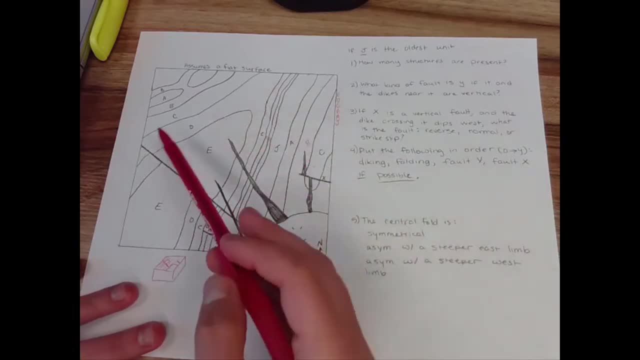 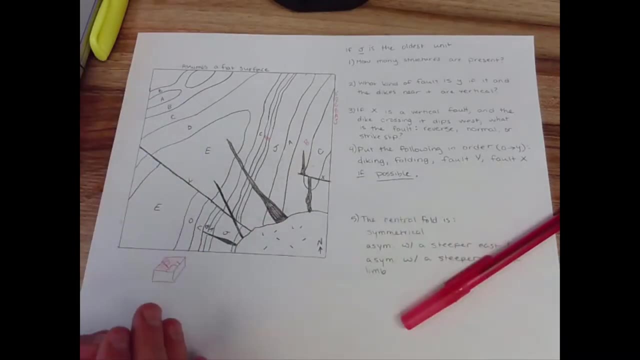 because it's kind of got this elf hat looking shape to it. when you have a fold and the youngest unit is exposed in the middle and it's and it's eroded down, the only way you're going to get that is by taking the top and going to the bottom of the unit and the left and right unit and the left unit. 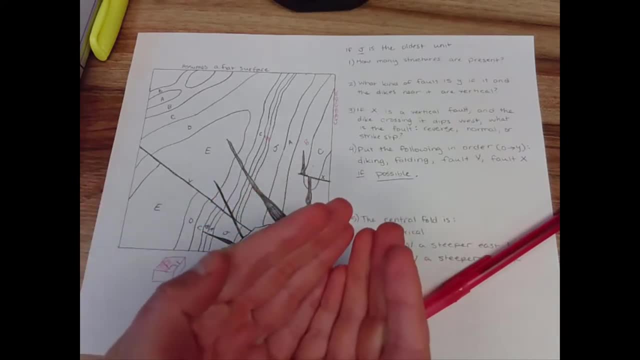 and the right unit and the left unit, and the left unit and the left unit and the own. only way you're going to get that is by taking the ground and curving it up and then eroding it down. So if I had, I could imagine taking Play-Doh in my hands. 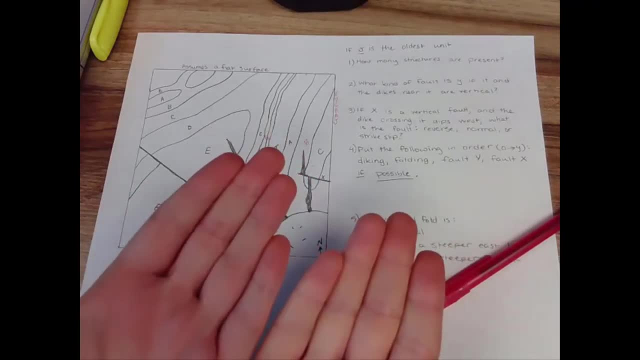 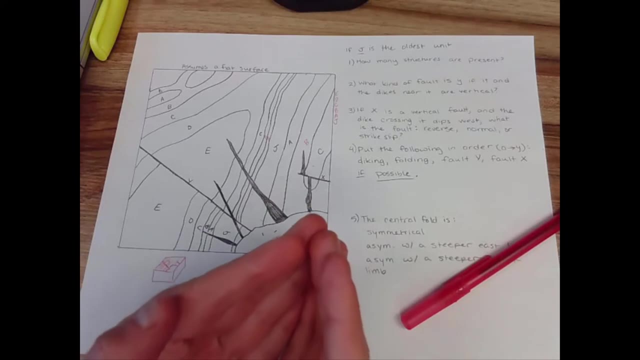 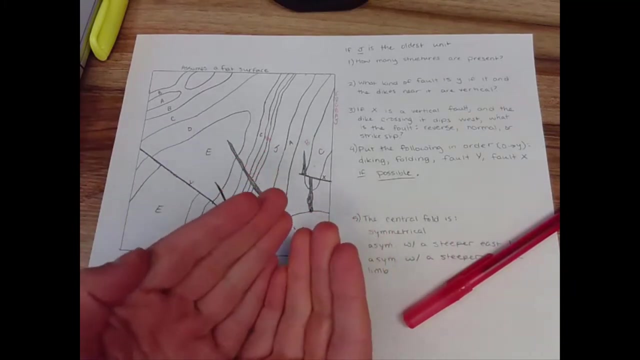 like this, and if it's deposited flat on top of my hands when I curve it up, that inside deposit is going to be present inside of the fold. So we've got one big fold here and that fold because it's curving up. it's a syncline. 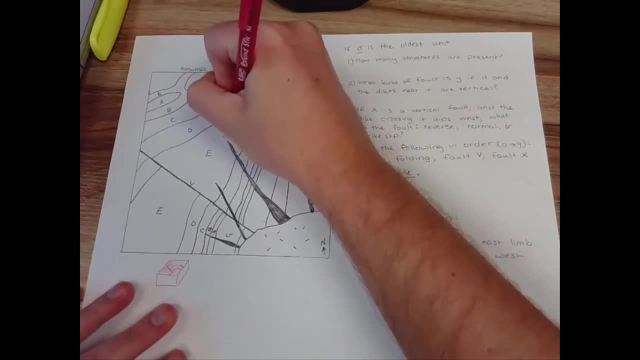 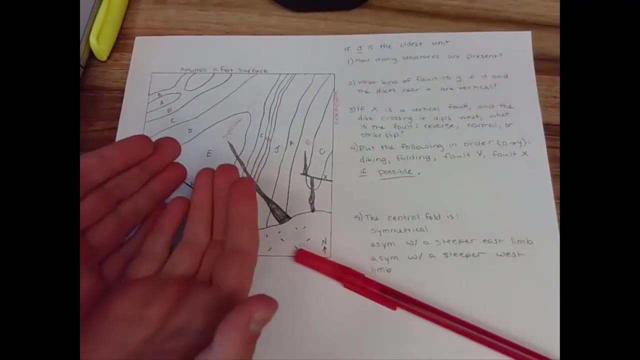 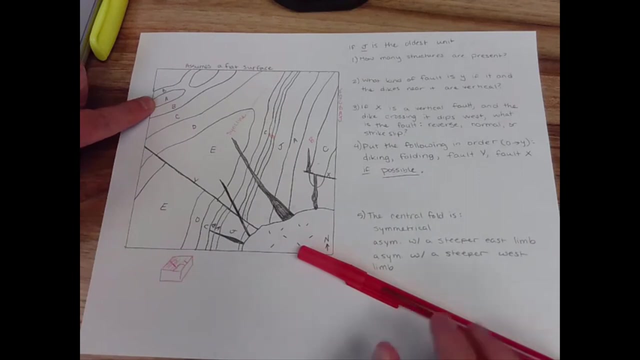 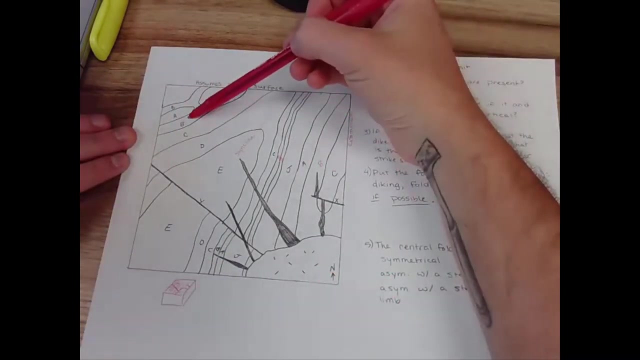 So I'm going to label this syncline kind of running down its hinge, and then, as it curves up, notice that over here it seems like we get older units exposed in a fold. So this is going to curve up and then this B must curve back and over here. 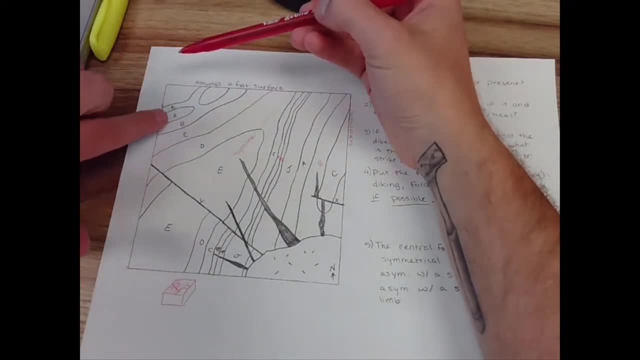 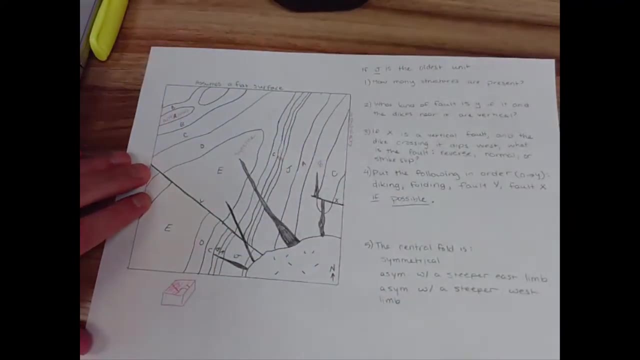 So it's going to make kind of like a little curve. It's going to make a little rounded top here and that's an anticline, Anticlines. you can tell because the oldest material is exposed in the hinge and then right here. 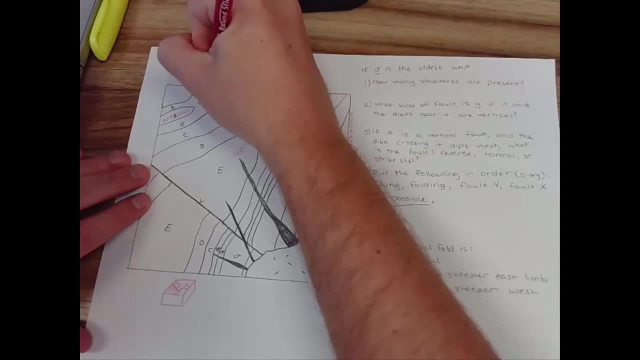 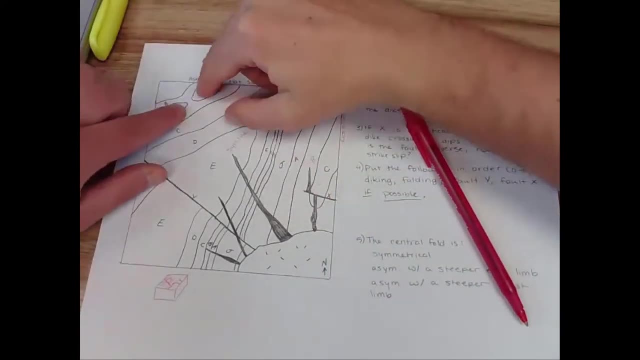 you've got it coming back this way. This is another anticline, just like that. Okay, so we've got two little anticlines and see how these tips are coming down like that. So you can kind of imagine two little hills, a bit like that. 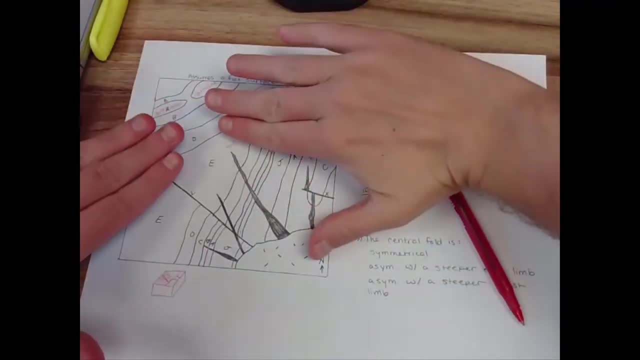 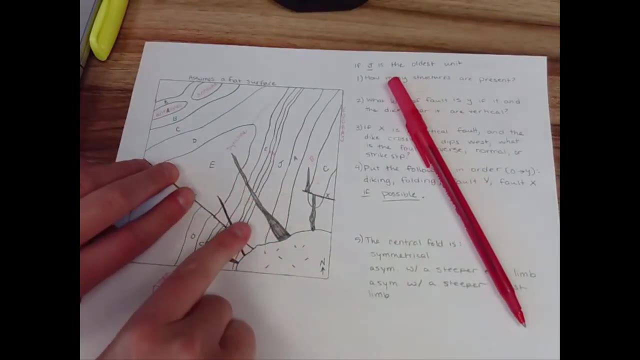 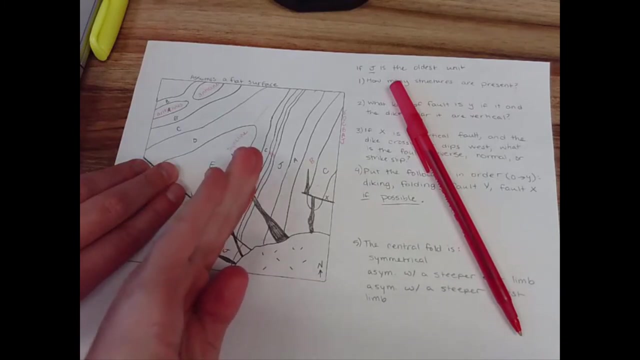 So two little anticlines we sweep into this big broad syncline and then right here these beds look really narrow. That's a trick of dip. So those beds are jutting up and you see how my hand goes from looking really wide to really narrow. 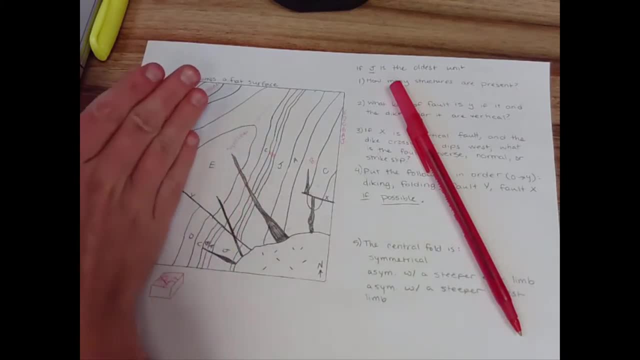 when you can only see the edge of my fingers. So that's a trick of dip, is that? this side of the anticline is broad and more sweeping, shallowly dipping, and then I rotate that limb up and it looks like that rotation. 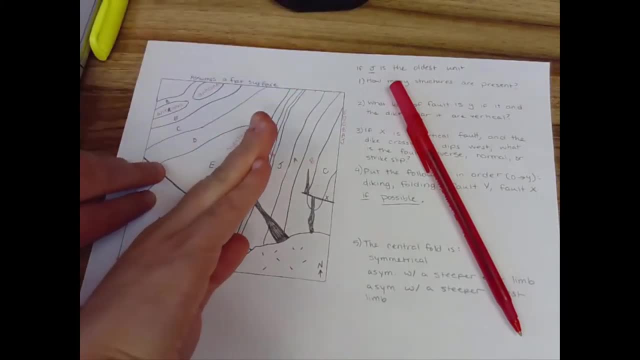 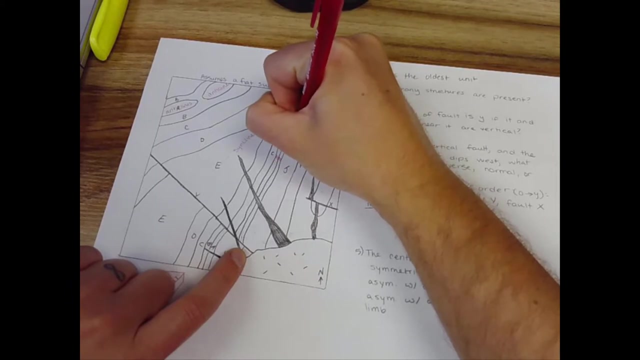 up is what exposes this oldest unit right here, which then curves back down and brings some younger material to the center again. So this, even though it's long and even though it doesn't look like it, this is actually an anticline. It's a long fold. 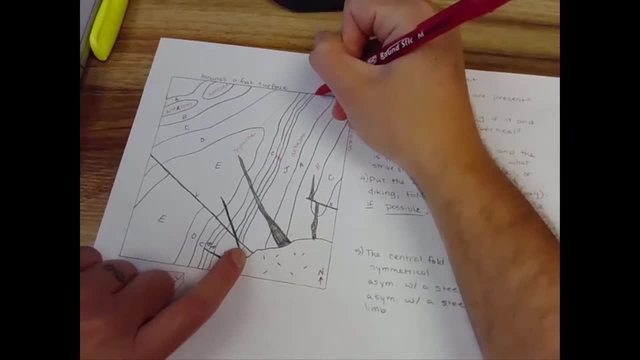 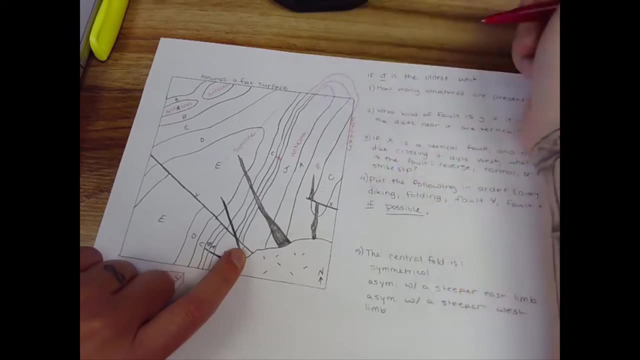 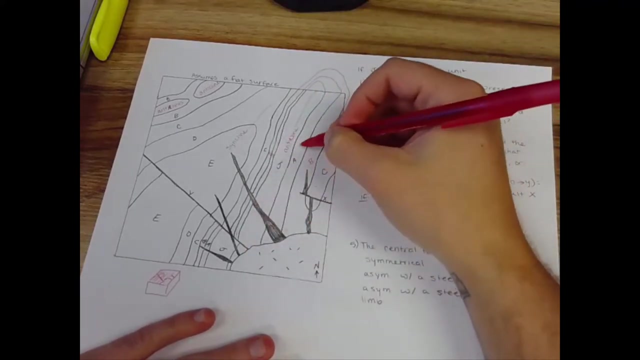 We just don't get a chance to see the tip, and maybe you know, maybe it's down here, Maybe it goes something like that, and we just don't get to see it. okay, So that's your anticline, So that's another anticline, and then we come down. 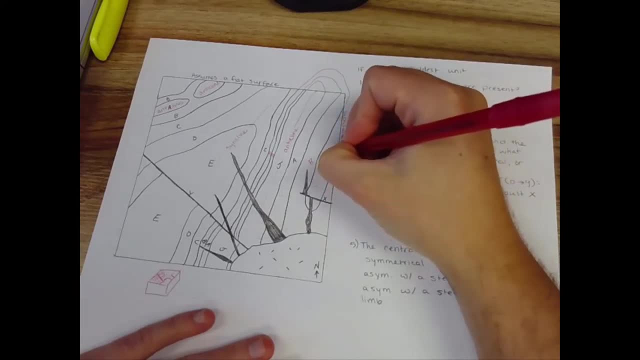 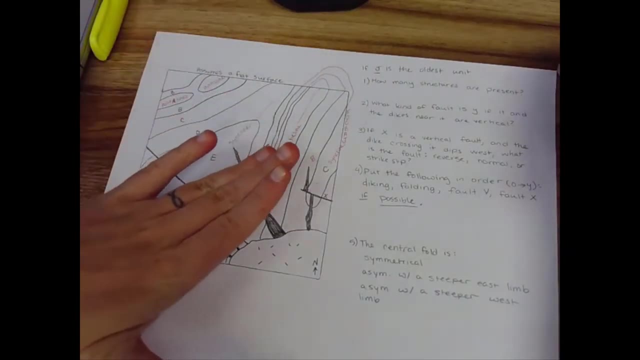 and bring this into another syncline. All right, so that's actually quite a few structures in there. You've got anticline, big, broad syncline with a steep dip on this side, a really sharp rollover of that anticline. 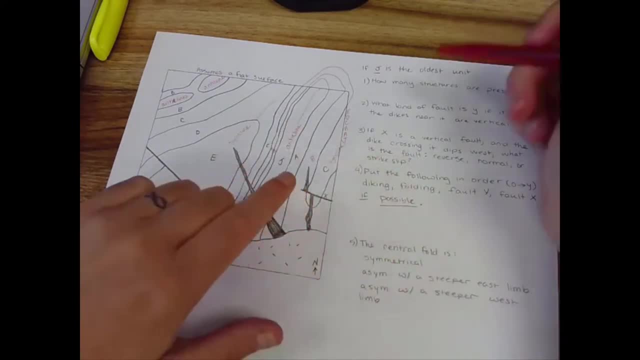 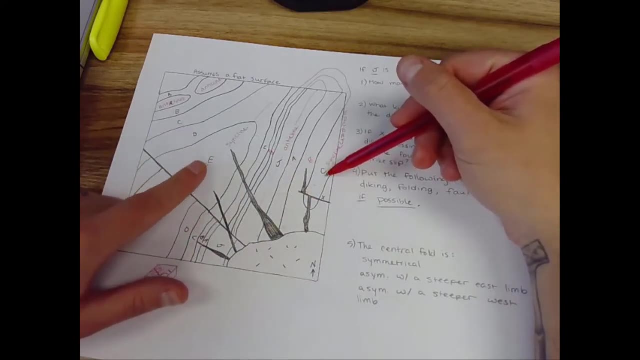 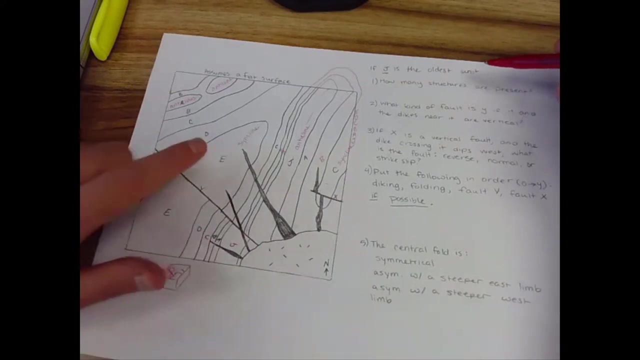 and now we're down into another syncline. notice: for this syncline, though, we're not exposing the same young layers as we did over here, and that's fine. there's no rule that says in one area you have to erode to the same, the same surface. 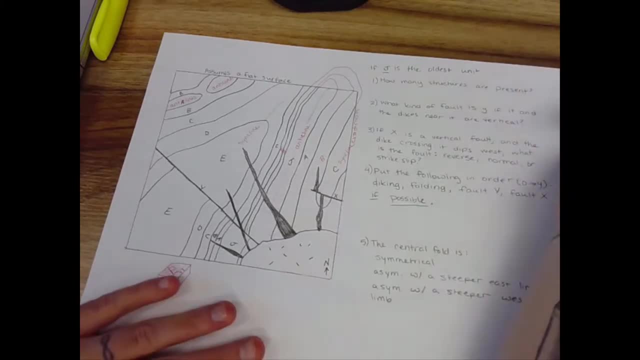 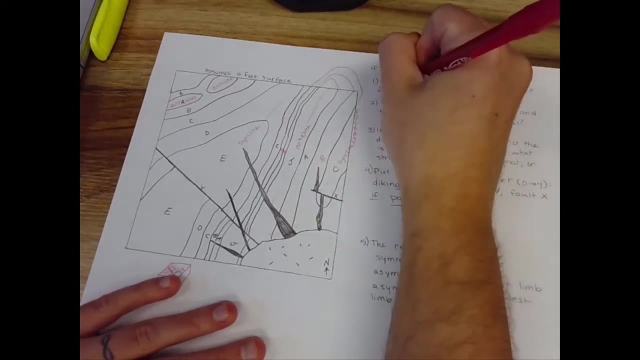 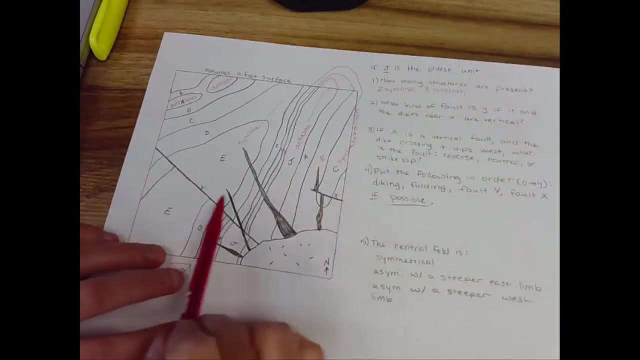 folds are allowed to be a bit wonky. so how many structures are present? there is one, two synclines, and there's also one, two, three anticlines. I see two faults, this one and this one, and these are dykes coming out of some kind of igneous. 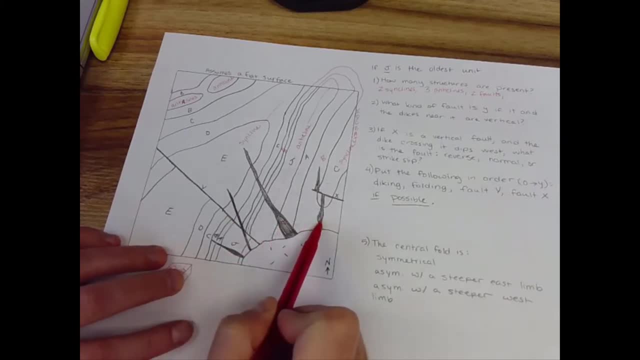 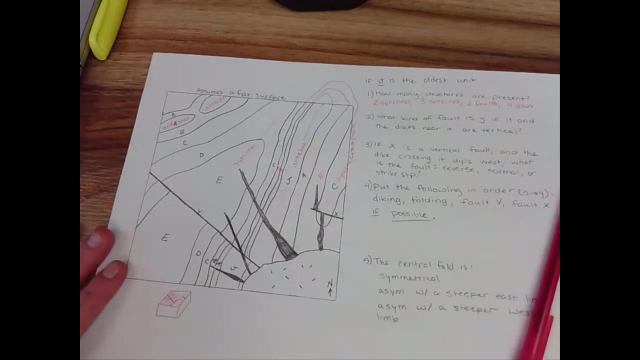 body. so one, two, three and fourth, that's offset for dykes. dykes count as structures because essentially they are filled fractures. alright. what kind of fault is why? if it is, and the dykes near it are vertical, and I didn't really mean, what kind of fault is why? I really just mean which side dropped, which side came. 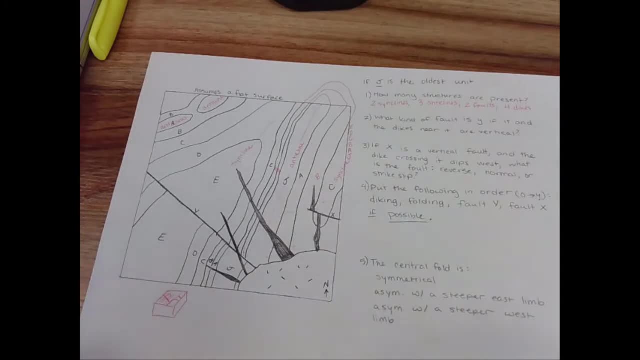 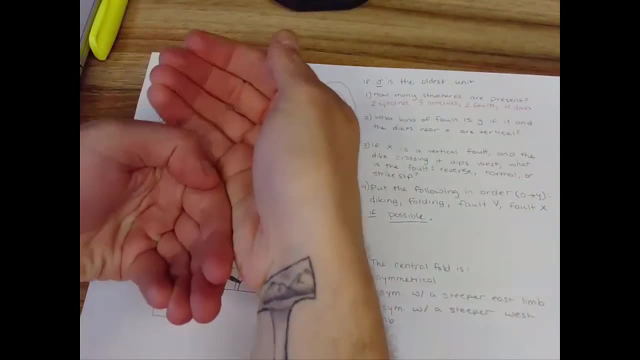 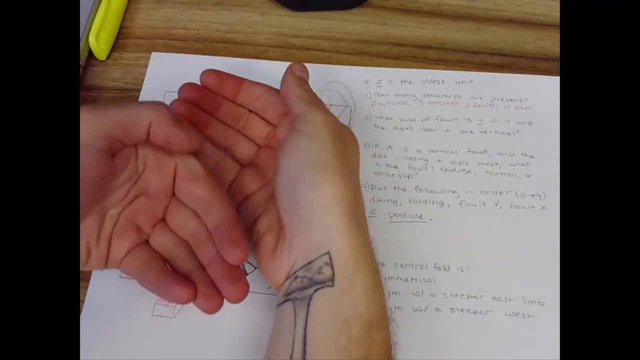 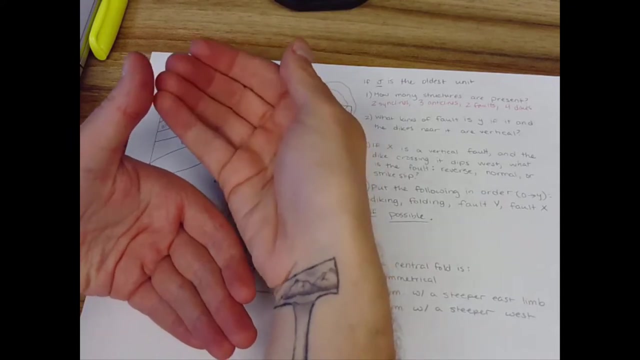 dropped down or which side moved up. so let's give our hands the data and take this by heart and use it as a useful tool for our project. okay, once again, if you've noticed how small the distance is, particularly like in---- in Safari, which you need a little space with it, right? so we're virtually 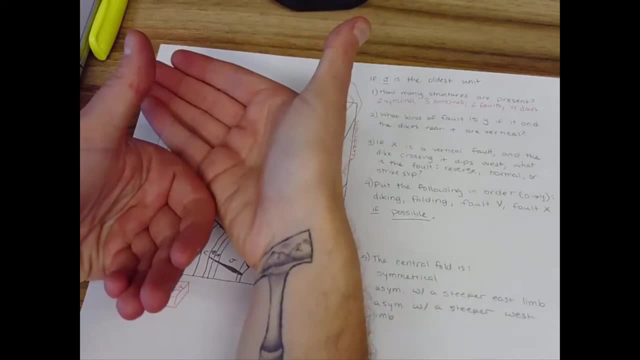 Santos, right, so you're probably thinking no, two flat on either side right here, and we're actually going to use this to estimate how big of a gap would be in the symcl weeks, or three, yes and a half area. where is this? if So, this means that the� 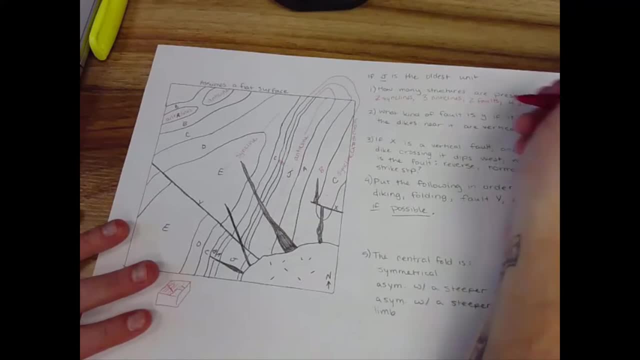 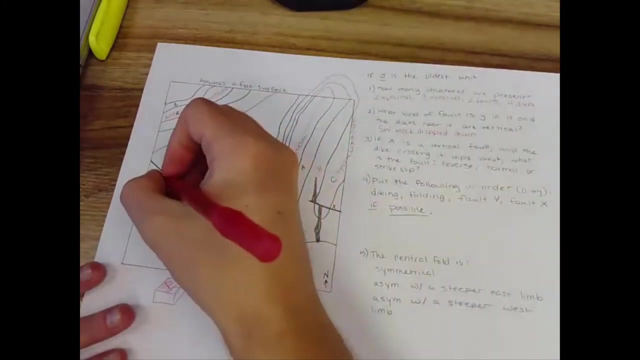 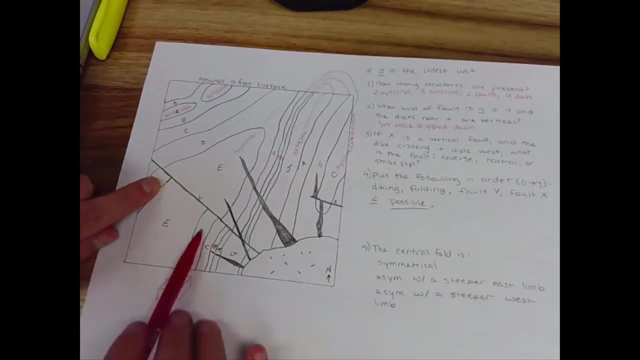 For Whoa形 periods are justified As this define sign guys then representắ� down. so I'm gonna put instead the southwest block drops down. okay, and that is really important to think through because a lot of you won't have necessarily seen a situation like this where a formation can look narrower on. 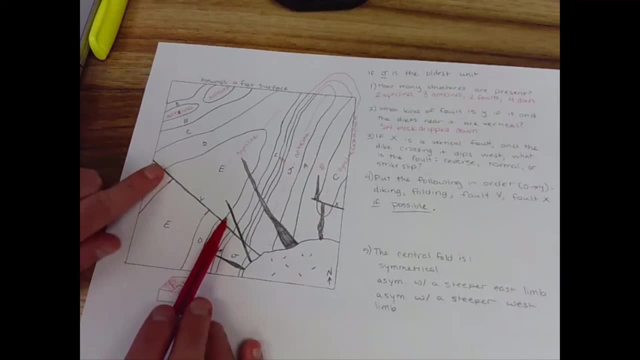 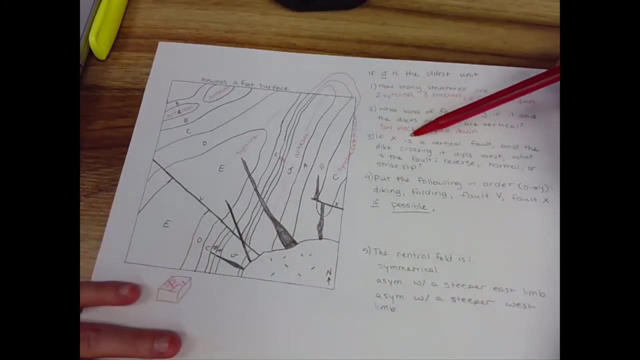 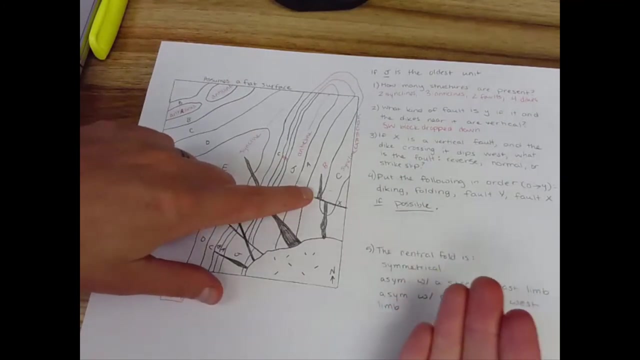 one side of the fault than it can another, and that is not due to any kind of weird offset, it's due to a vertical offset plus erosion. right, if X is a vertical fault and the dike crossing it dips west, what is the fault? reverse normal or strike slip, okay, so the fault is vertical. and again this, I'm so sorry. 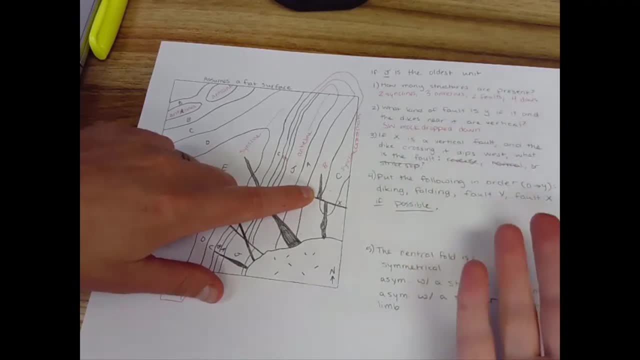 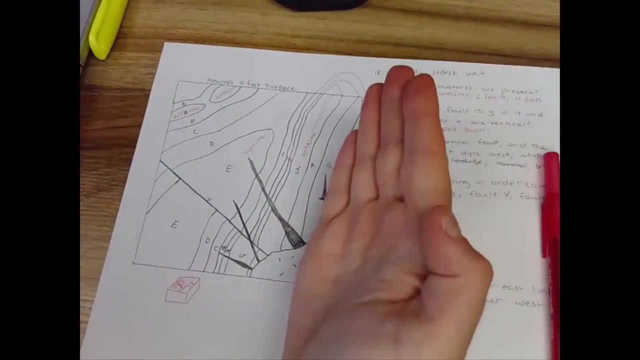 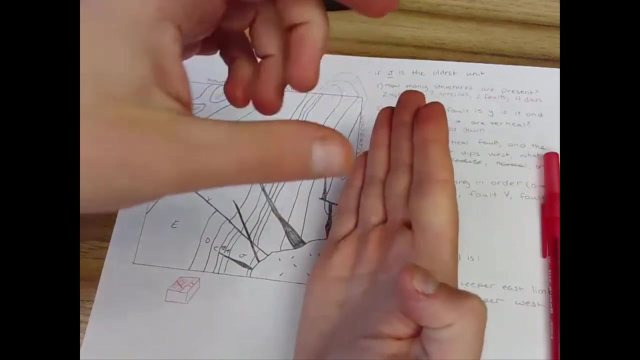 about the way I wrote this. let's just decide is it strike slip or not, and if it's not, which side which block drop down. so if I have a block or if I have a dike dipping like this and I have a vertical fault crossing it like that, let's practice sliding each side. 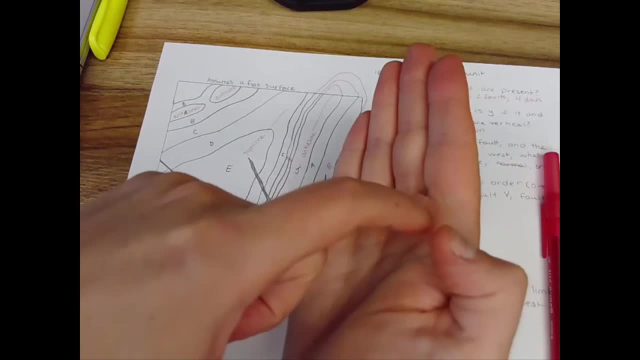 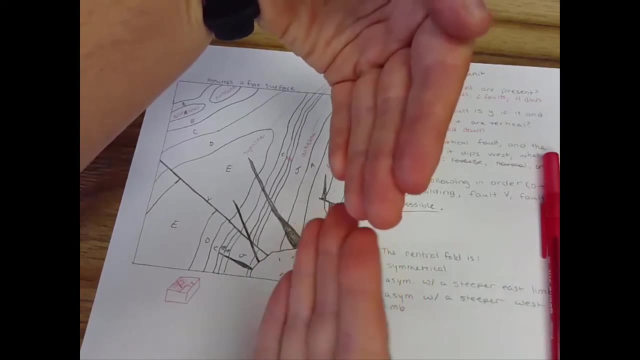 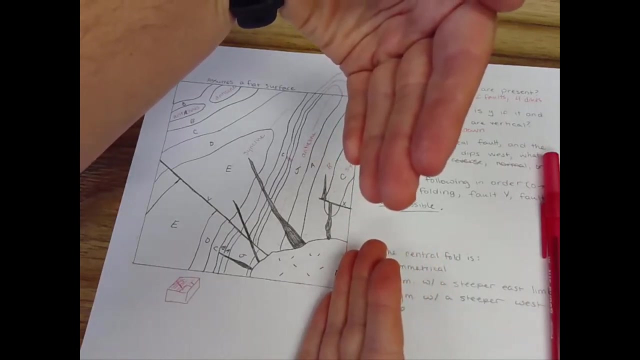 down and see what happens if this side slides down before, before faulting, we're gonna say: the rock is dipping like this, we're going to let this side drop down and then we're going to erode this down to the surface where this dyke, this side of. 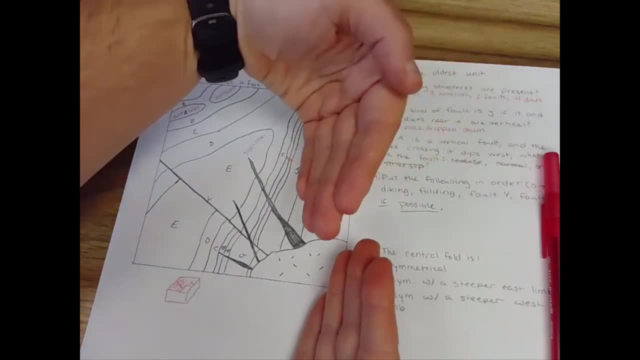 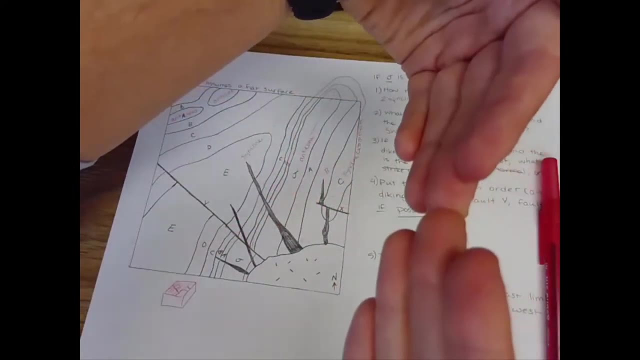 the dyke ends up being exposed is going to be out here. okay, now let's see what happens if we drop this side down. if we take this side of the dyke and we drop it down, when we start to erode this one, we end up yourself between both of them. we end up on the opposite side. okay, now what happens? if we take the bottom end, we make this one the first one, and when we start to erode the first one, we end up on either side. we end up off to the side and sort ofонов macrame, and then 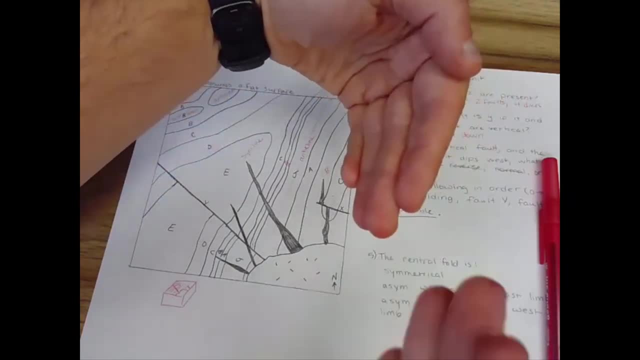 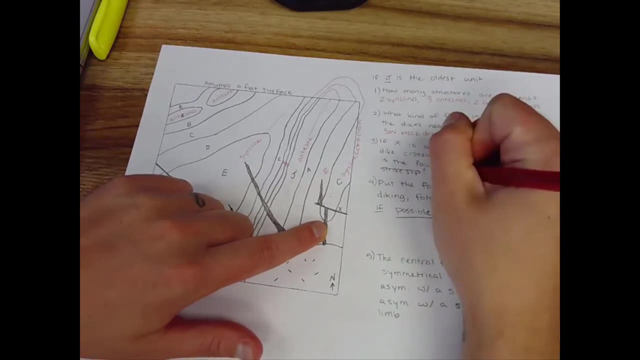 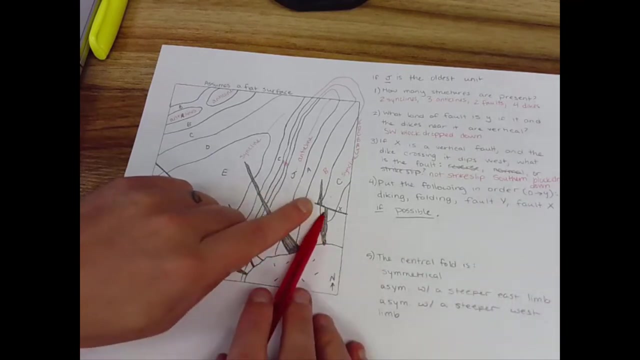 we you're going to want to funded off of all the ceiling shapes, but when we start, end up with this block in front. so this block has to be the side that dropped down. so the southern part dropped down. it's not strike slip necessarily. and the southern block dropped down. here's what I'm saying. this is not strike slip, I'm. 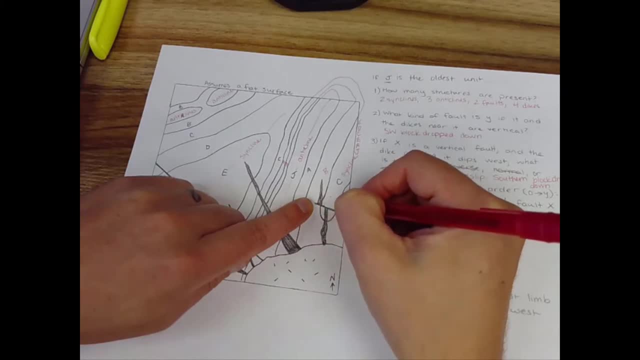 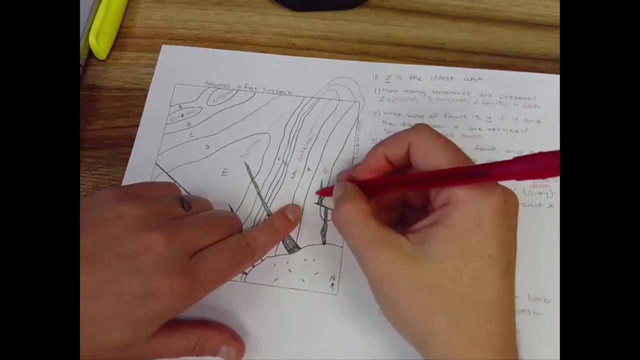 saying that this is not strike slip, because it is clearly cutting across this fold, but it is not offsetting that fold. if this had been strike slip, we would anticipate this fold to be offset in this direction and it's it's not okay relative to this part of the fold that's preserved on this side of the fault. so 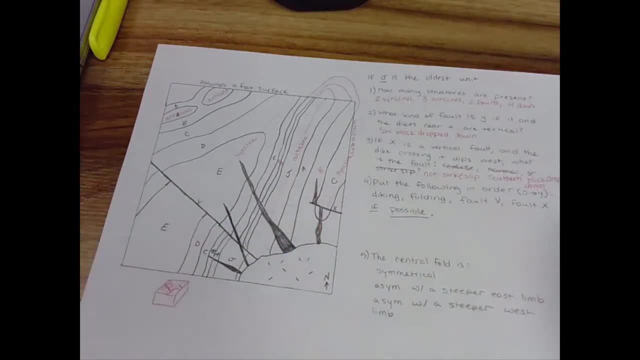 not strike slip. the southern block dropped down. now let's put these in order from oldest to youngest: dyking folding, fault Y and fault X, if it's possible. so for me I'm gonna check out this folding first, because it seems to impact the largest area. I have folds cross, cut by faults. I have folds cross. 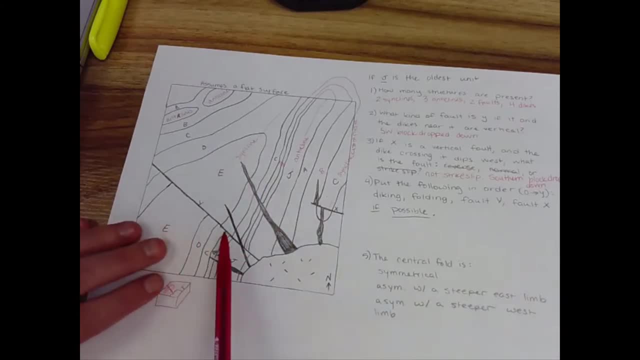 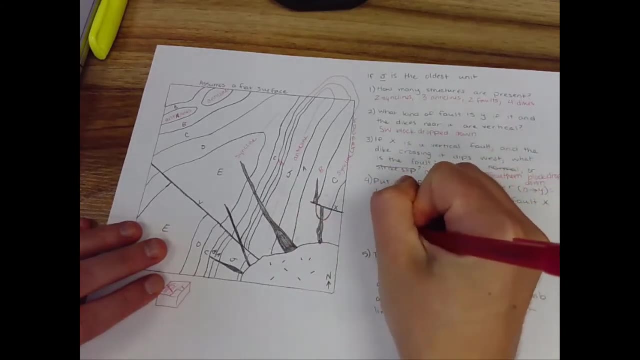 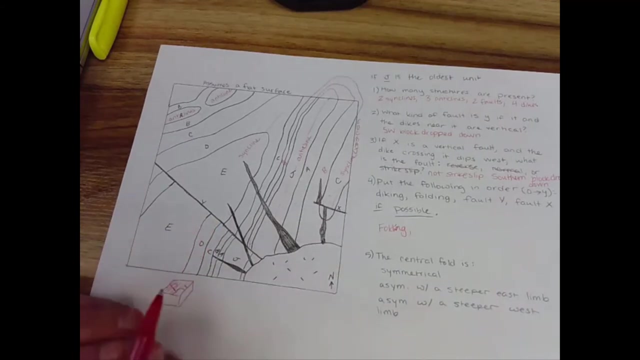 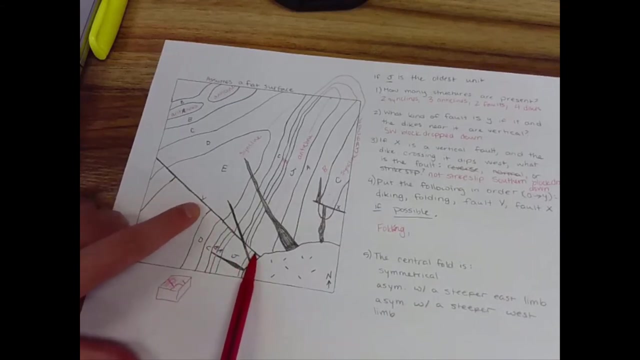 cut by dykes, 三項. so, and also over here the folding is cross cut by the dyke. so the folding is going to be the oldest folding, oldest thing we have here. then what's older, the dykes or the faults? so here are on fault Y: 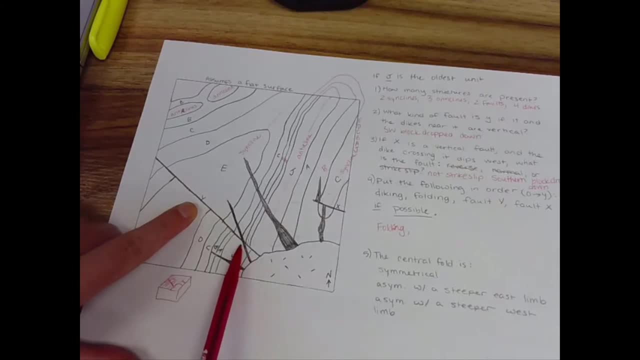 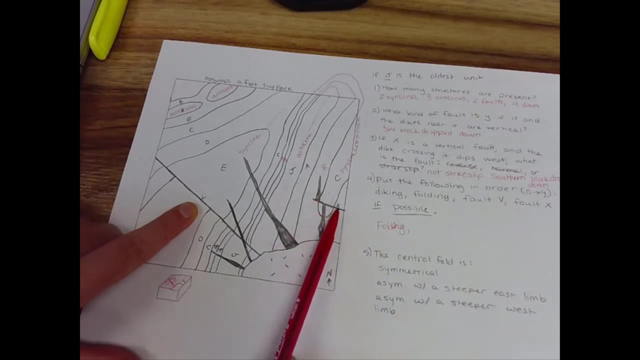 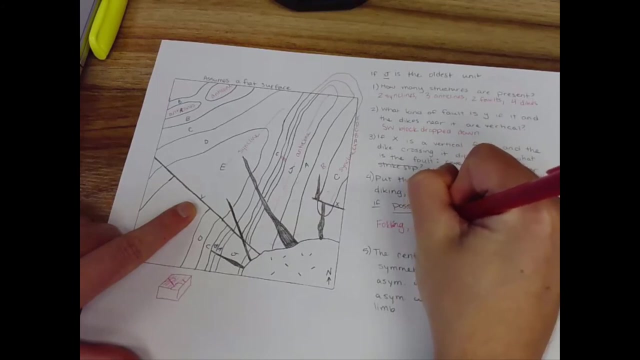 I really can't tell if that dyke is older or younger because it's vertical. But here, with fault X, I can definitely tell that fault X comes after the dikes. So I'm going to say diking or fault Y And the last thing is fault X. 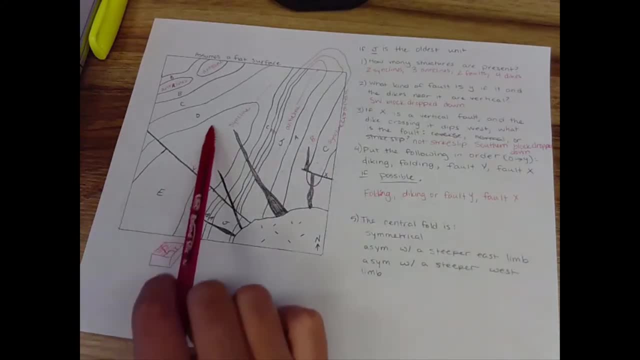 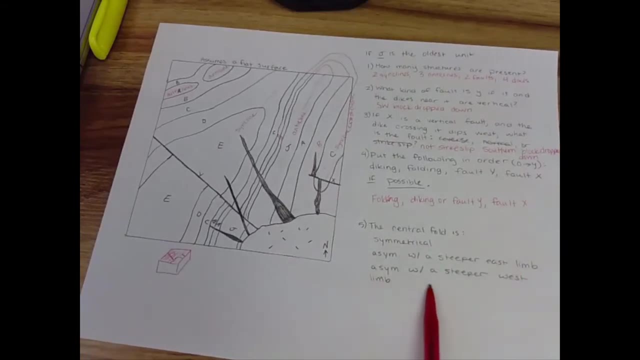 All right. last thing, here, the central fold. So that's this thing. right here, The central fold is symmetrical, asymmetrical with a steeper east limb or asymmetrical with a steeper west limb. So give yourself a sincline. 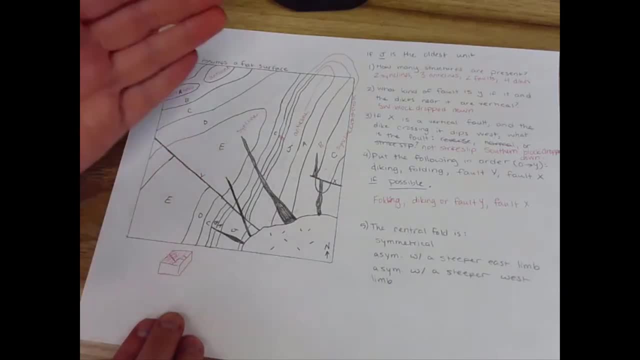 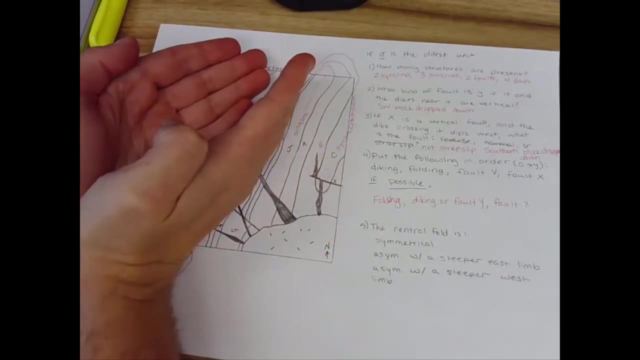 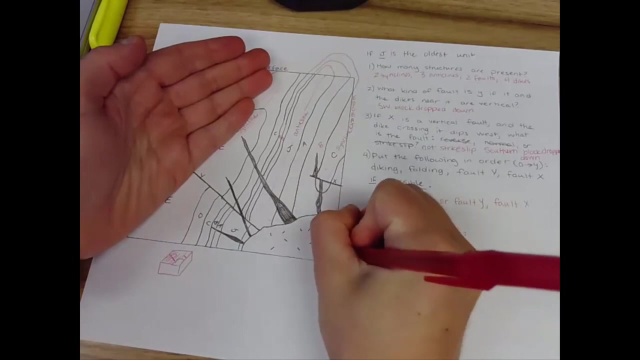 On this side the beds look thicker, so they have to be shallower dipping. On this side the beds look thinner so they are steeper dipping. So over here, your east limb, because this is north, this is west east. 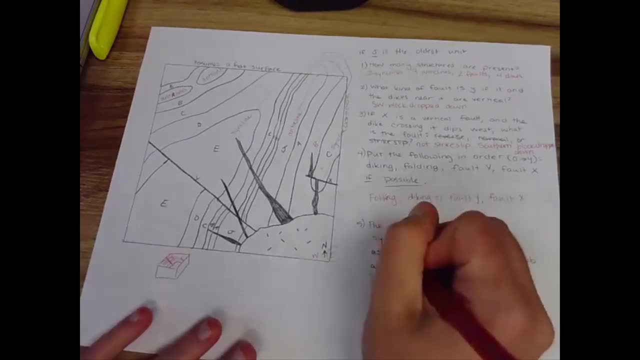 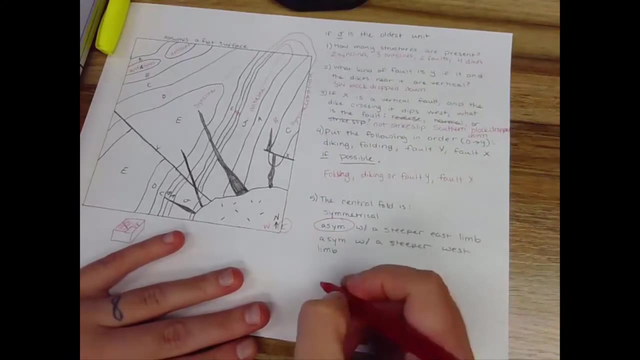 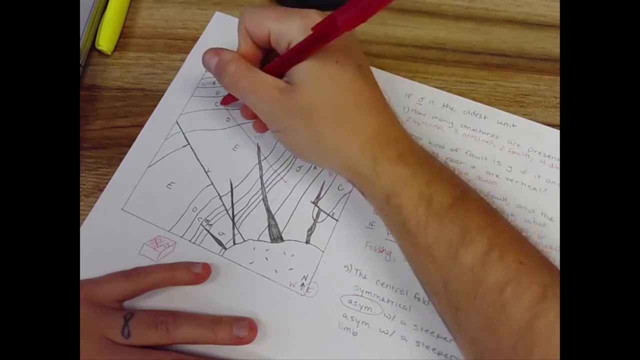 your east limb is steeper dipping and it's asymmetrical. So if that wasn't entirely clear, let me just draw a quick cross-section. And I'm just going to draw a cross-section from. let me do one from C to J. 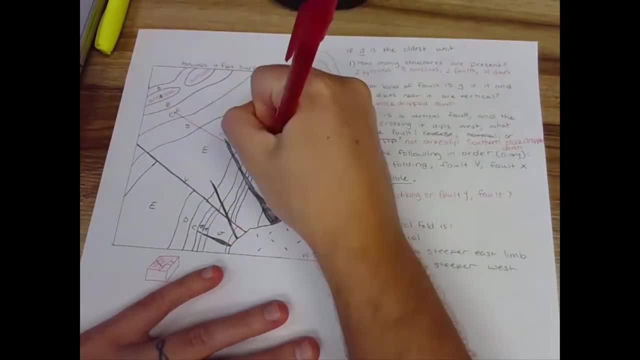 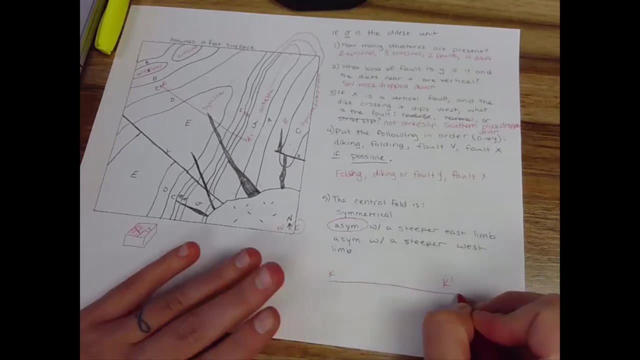 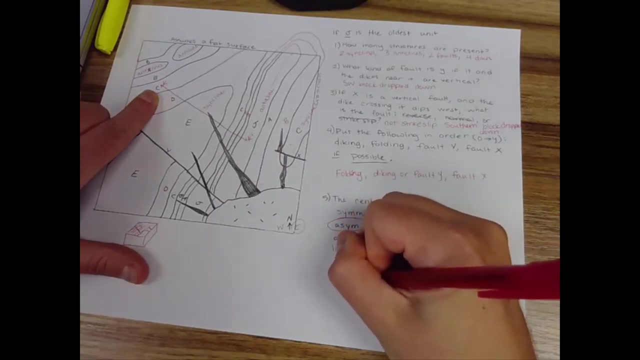 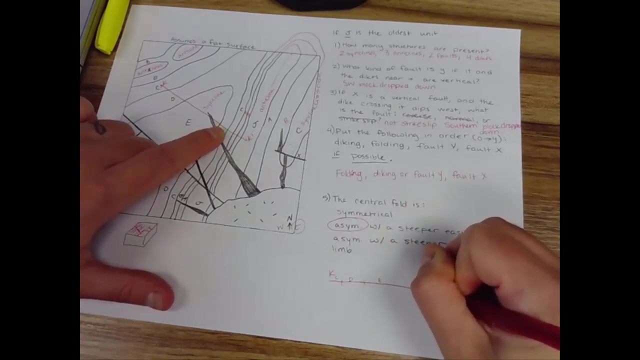 We're going to call this K and K prime. Okay. So we've got topography, which is great. We've got C, D, a big section of E, then D, again C, again B and A. Okay. 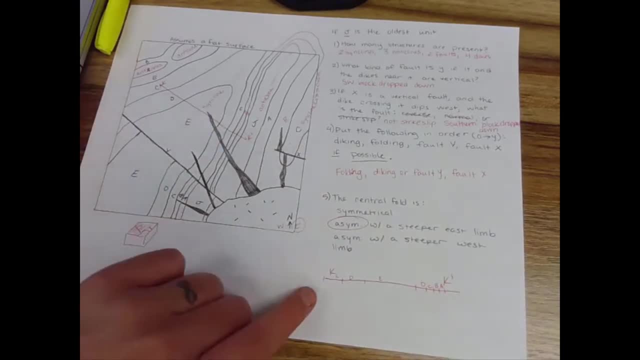 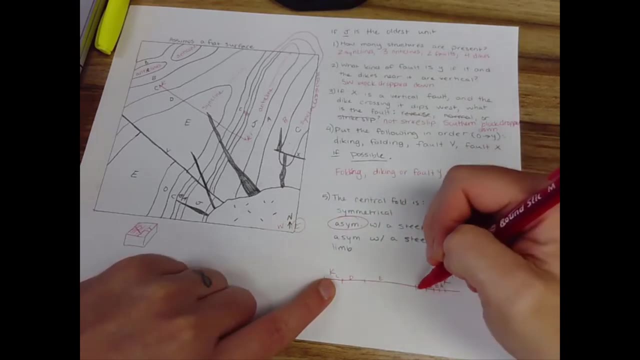 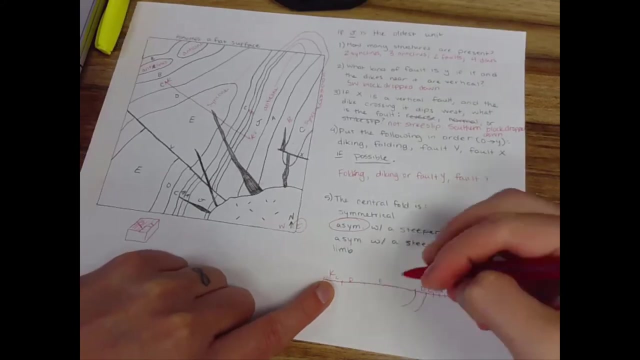 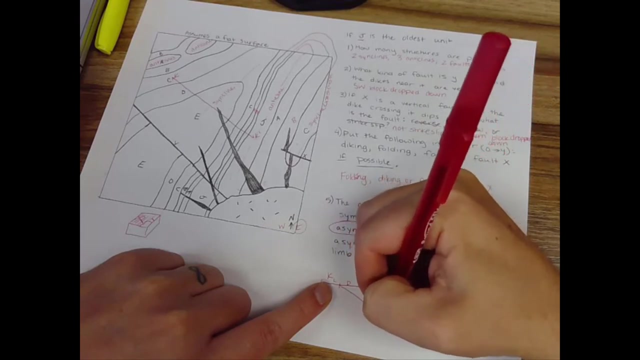 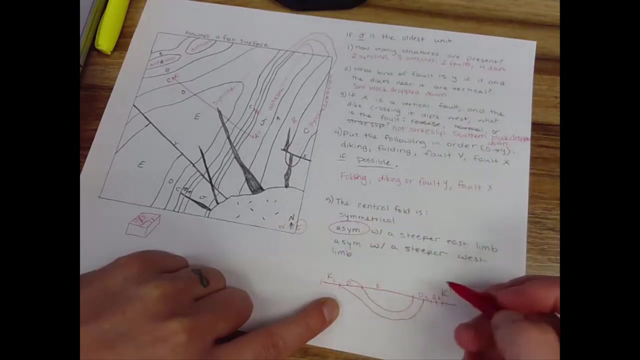 I'm going to go a little bit farther just to capture all of C. So check this out. If I try to connect D and D, the only way to maintain bed thickness is to bring it like this, And I drew a little bit above the ground just so you could see this thickness. 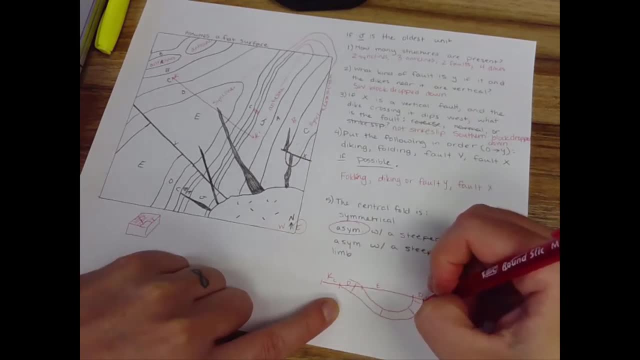 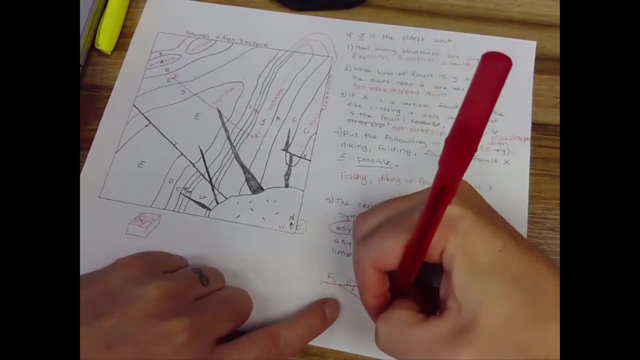 and I didn't draw a cross. Okay, So this is the same as all of these thicknesses through here. So C, let's do this the same way. trying my best to maintain bed thickness, I've got to shallow my bed out right there.